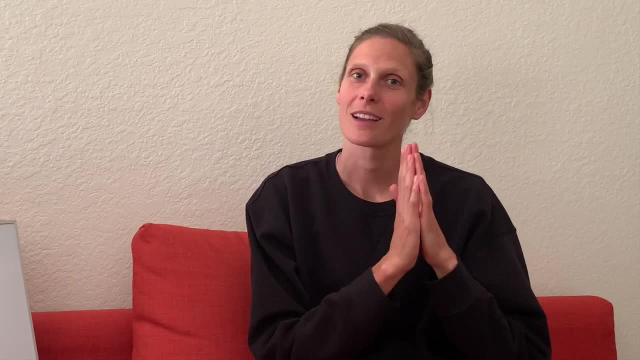 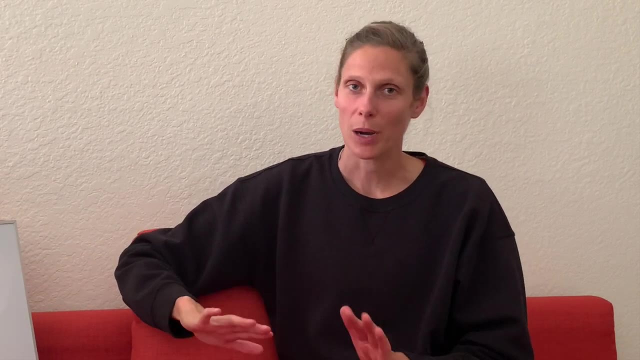 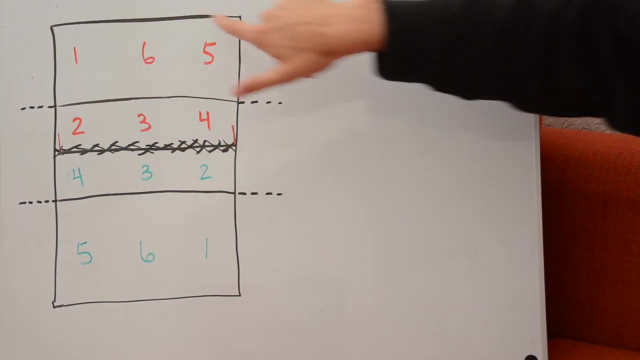 Knowing the serve receive formations is a whole other video and a whole other issue. So for now we're not going to get into that. But the important thing is that before the serve every single player needs to be in this orientation and in this position relative to the other. 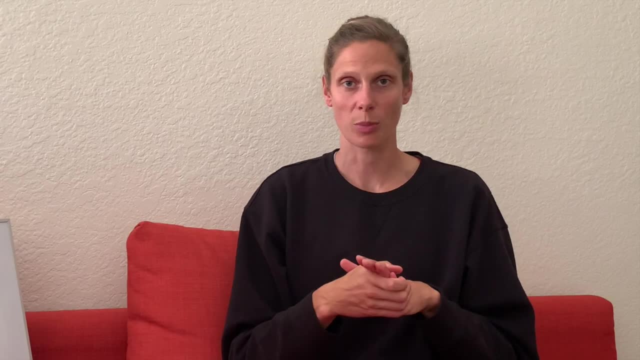 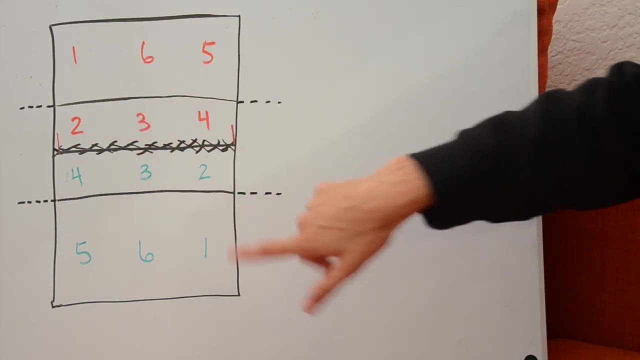 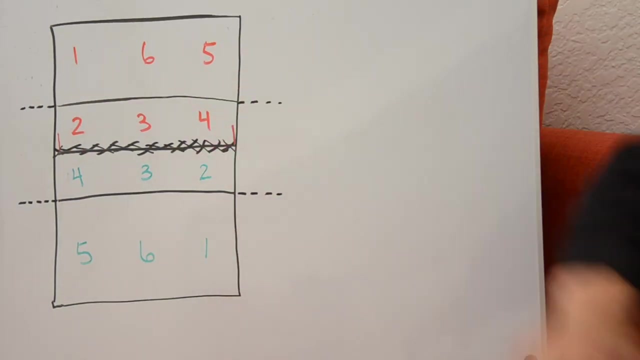 players on their own team. Once the ball is entered into play, players can move anywhere on the court. These numbered positions and delineated areas are only applicable before the serve happens. Player number one is going to serve the ball to the red team. Everybody's in their position and as soon. 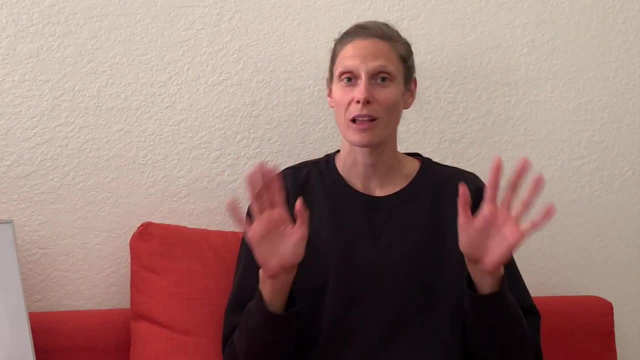 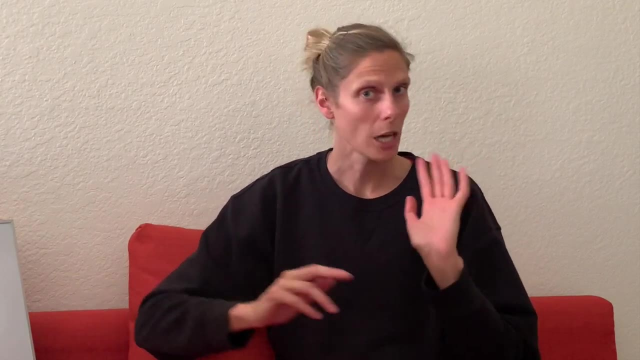 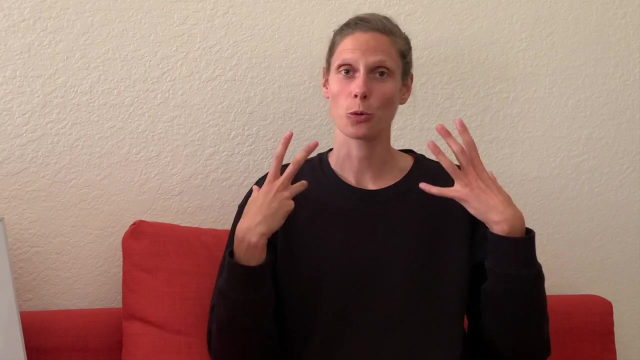 as the serve happens. everybody moves around and you play volleyball the way that you know how. if the green team scores, number one is going to serve again, and this continues to happen. whoever is serving, if you, your team, wins that play, the same person keeps serving the whole time. 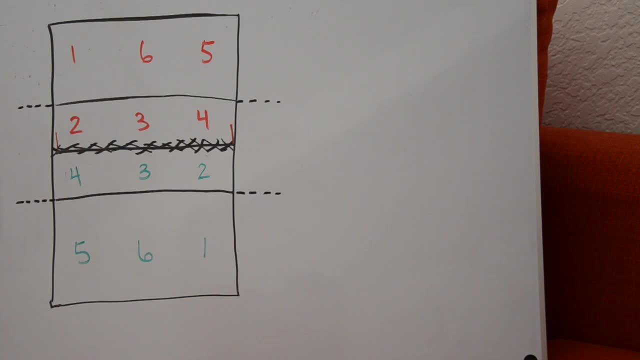 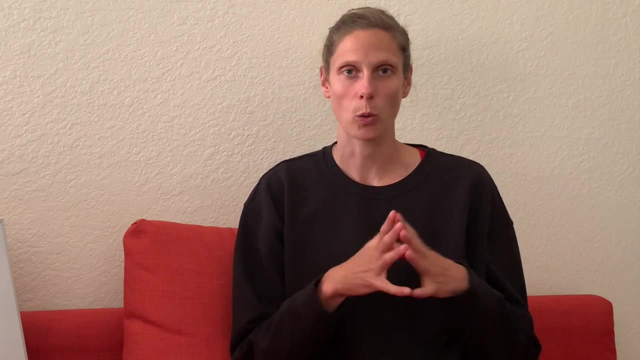 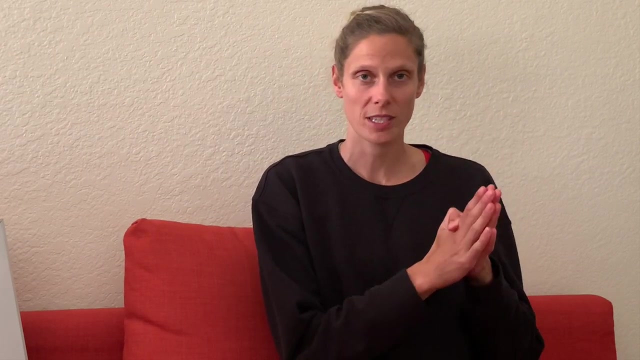 let's say that the green team loses the point. okay, so now the serve goes to the red team. if your team is on serve receive and you win the point, that means that your team has earned the right to serve when you transition from serve receive to serving. that is the point in time. 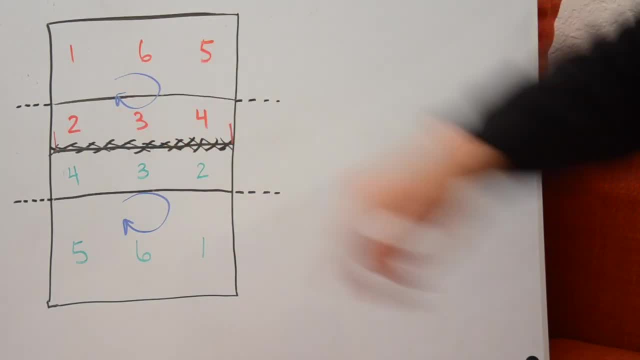 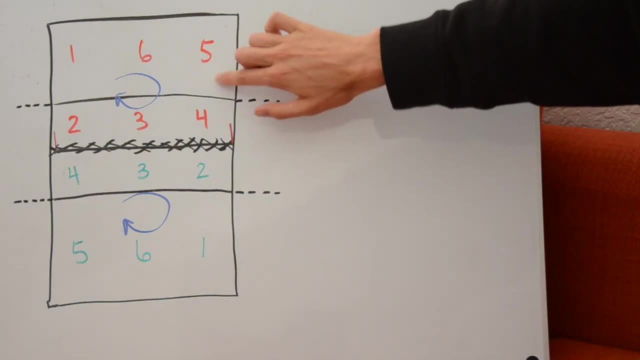 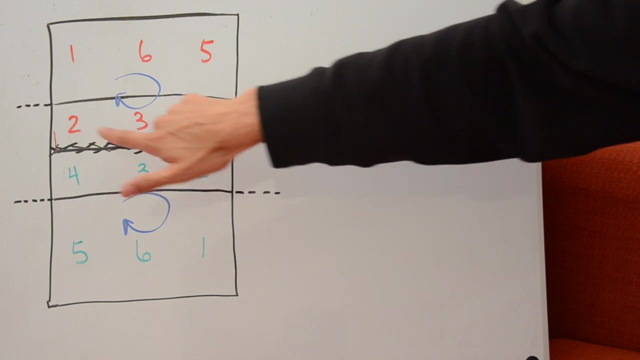 that your team rotates and you rotate in a clockwise direction. so in this case, when the red team earns the right to serve, the person in position two will rotate to the back. one will move this way and all the players will shift one position, meaning that number two is the next. 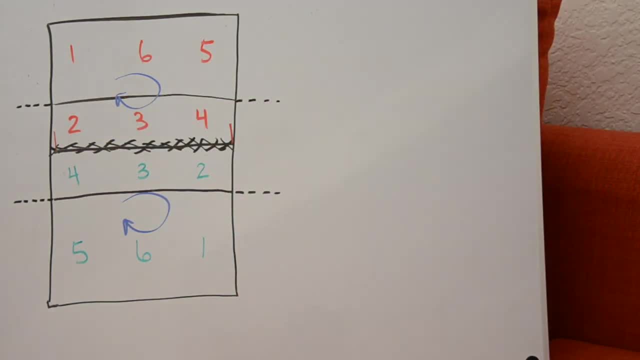 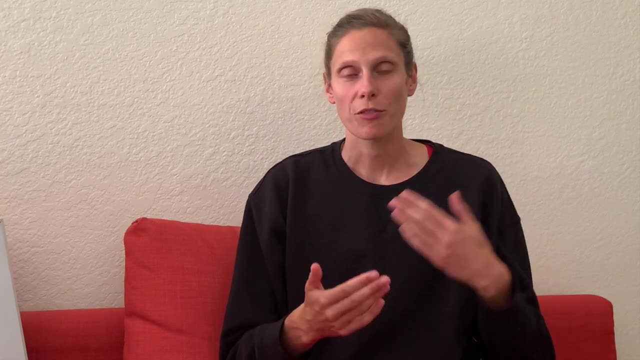 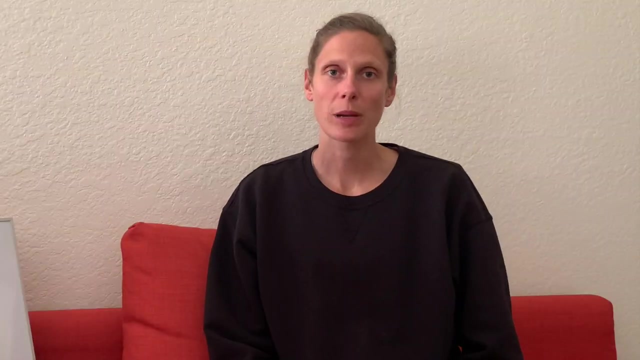 server The green team. on the other hand, the green team was serving and they lost the right to serve. If you transition from being the serving team to the receiving team, you maintain your position Because the red team has rotated and is now serving, but the green team has maintained. 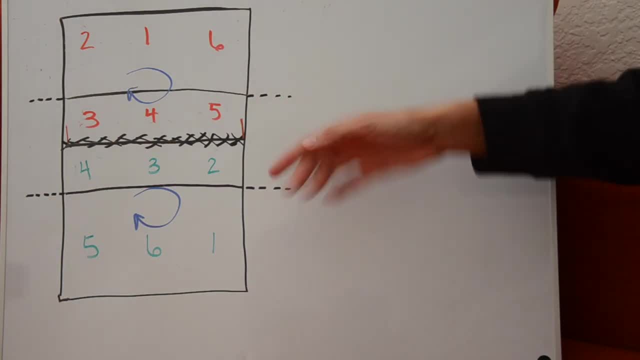 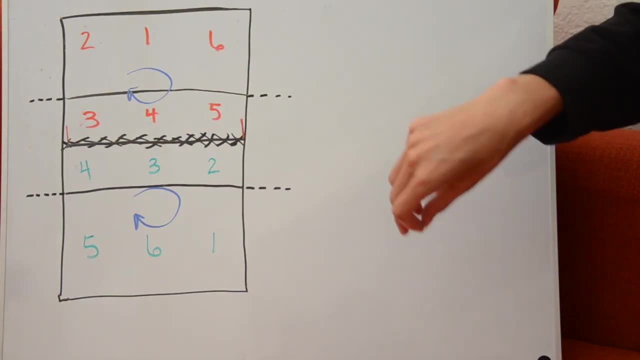 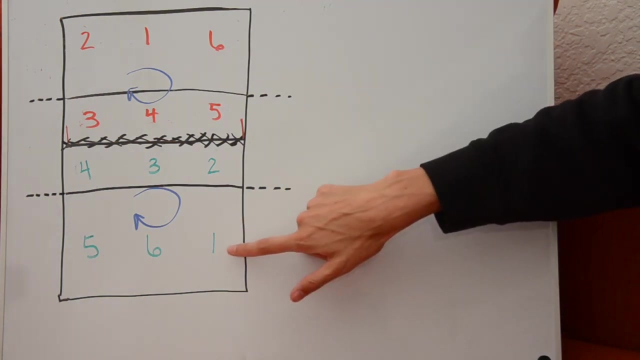 their position. this is what the new layout looks like. You can see that this team rotated, all of their players moved and number two is now serving. But because the green team lost the right to serve, they need to be in the service-y formation where they currently are. So that's why. 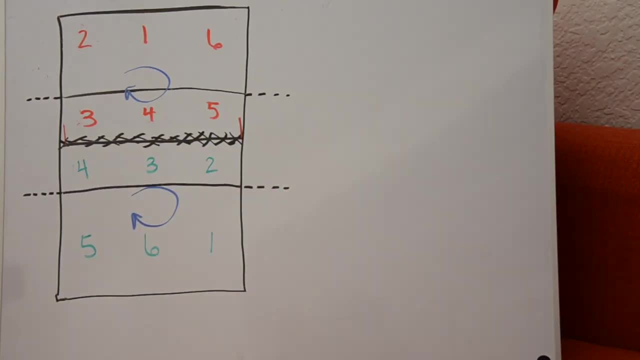 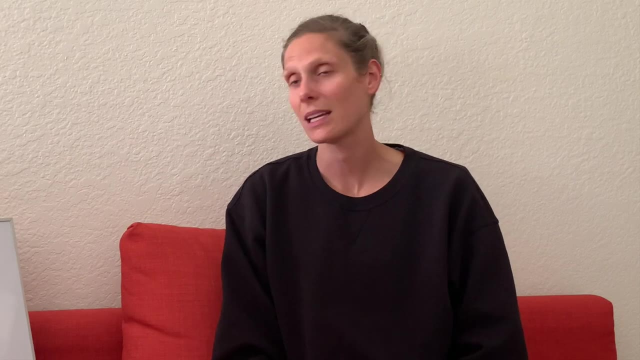 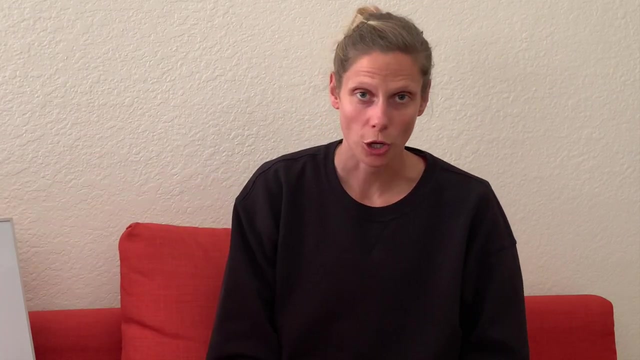 all of their players are now serving. All of their players are in the same position. So now number two is serving, The green team is staying in their service-y formation and play proceeds. Number two on the red team will continue to serve until they lose the. 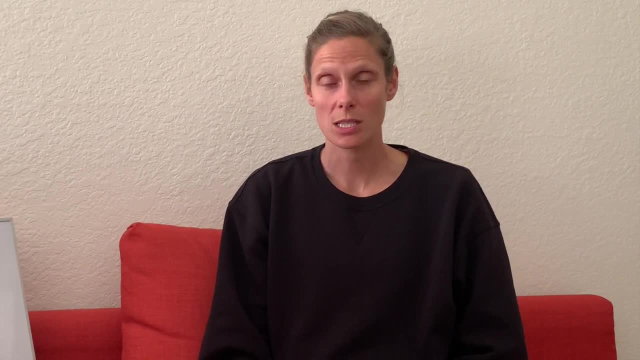 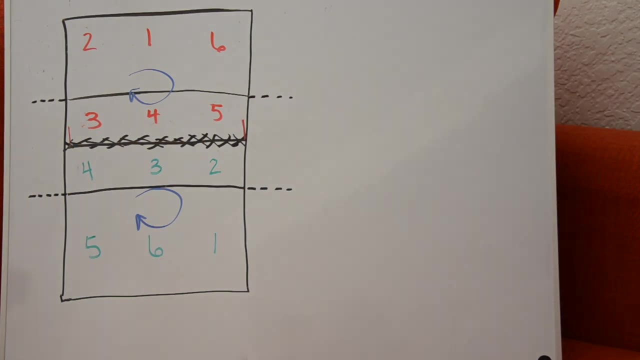 point. Once the red team loses the point, they will stay in this position and be in serve-receive. But because the green team transitioned from serving to being the receiving team, they need to be in the serve-receive, serve-receive to serving. that is when they will rotate. 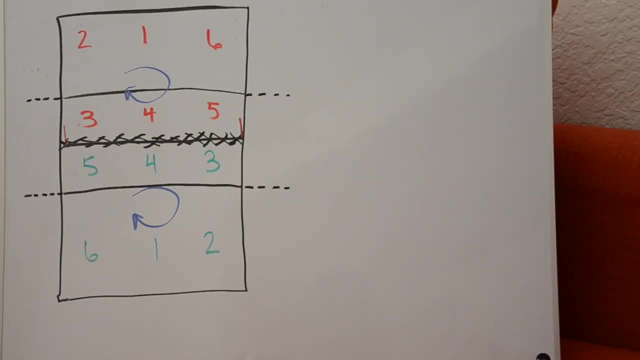 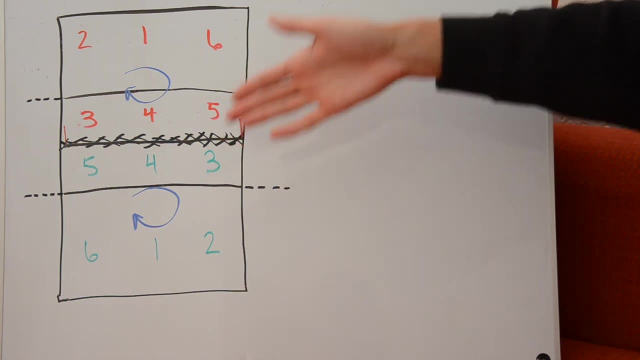 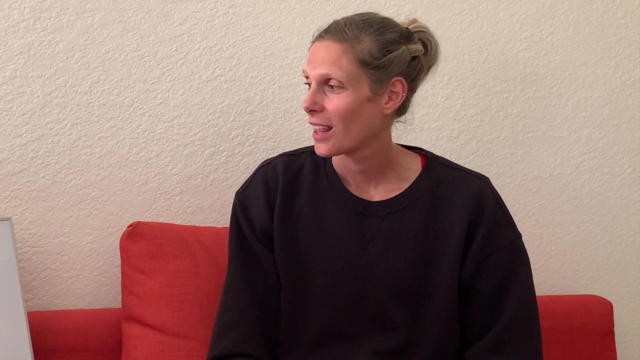 And here's what the next pattern looks like: Because the green team rotated and now has the serve, number two on the green team is the server And the red team moves back into their serve-receive formation from where they currently were. This will continue to happen for as long as the game lasts. 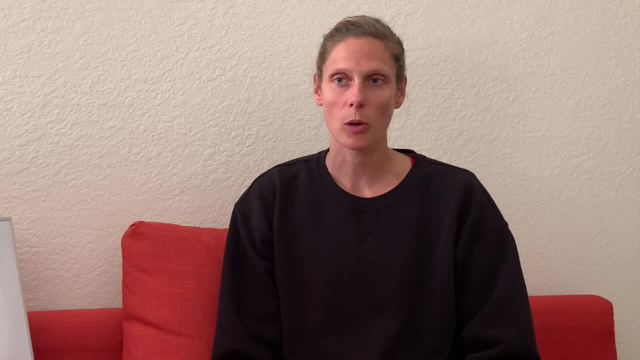 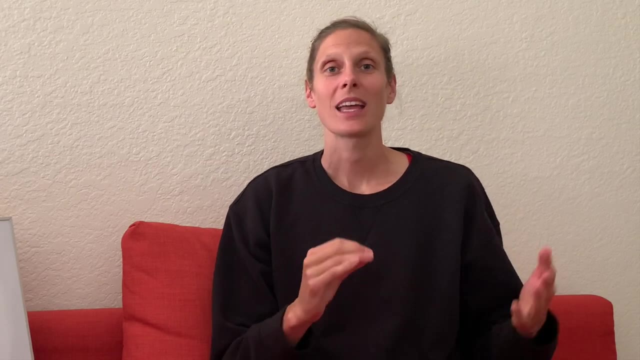 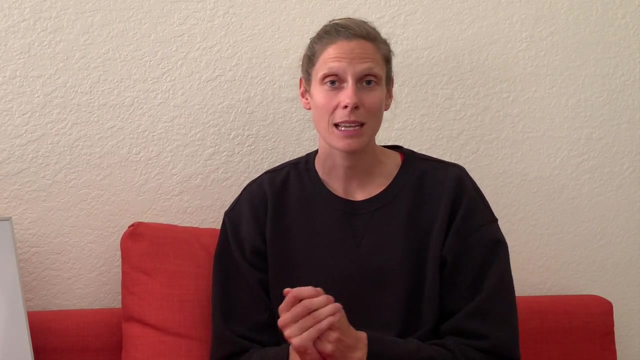 An important thing to know is that in indoor volleyball, every single time that there's a serve, one of the two teams will get a point. So if the server serves and misses the serve, the receiving team gets a point. If the receiving team goes up and hits the ball and scores. 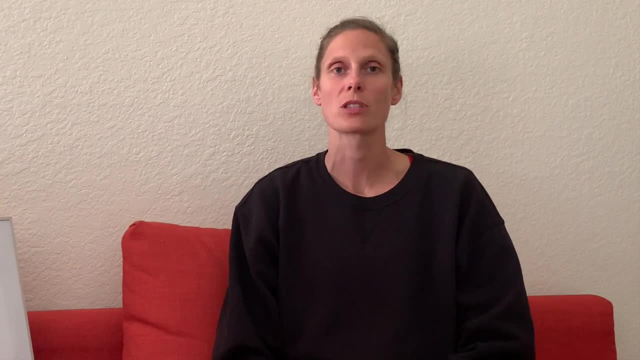 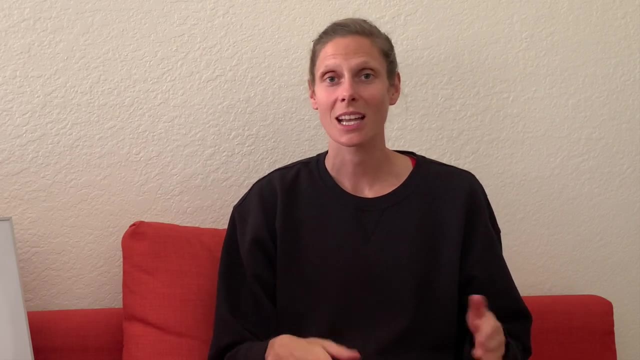 they get a point. So every single time the whistle blows for somebody to serve, one of the two teams is going to get a point. In indoor volleyball, the game proceeds like this until somebody reaches 25 points or until somebody is winning by two. So, for example, if the score is tied at 24-24 and somebody makes the score 25-24,, the difference in points is only one. So the game has to continue until it's either 26-24, or it could even go higher. 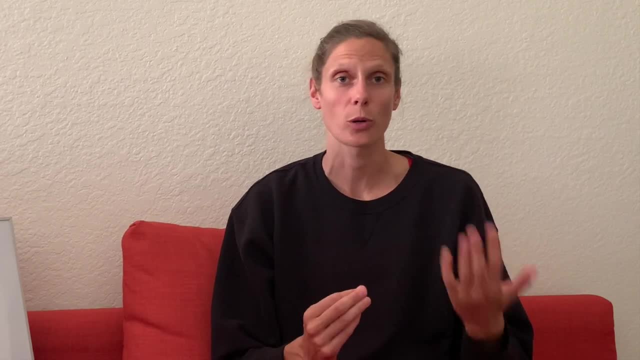 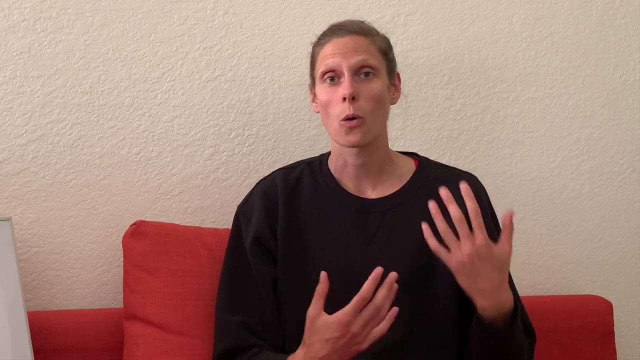 In the tie-break set, whether it's the third set you're playing two out of three or the fifth set in three out of five, the score only goes until 15 points or until somebody is winning by two. I hope that helps you understand a little bit.